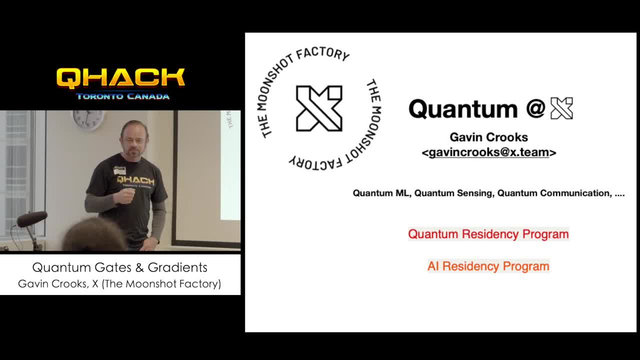 I mean right, And we now have a quantum group within X. It's relatively new and we are distinct from Google's, you know, hardware group, And so we're sort of doing the quantum things that aren't the quantum hardware. So we're doing things like looking. 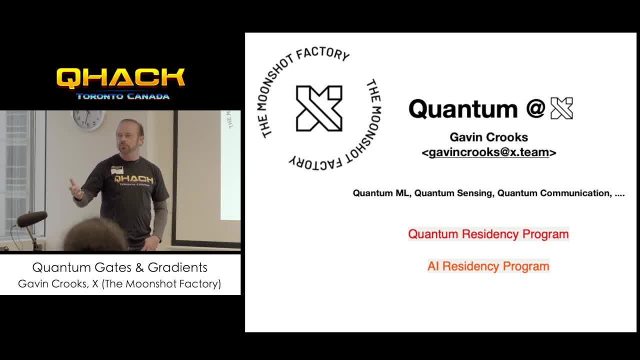 at quantum machine learning algorithms, but more broadly than just quantum computing, looking at things like quantum sensing, quantum communication. Lots of really cool things going on, most of which I can't tell you about right now. I just wanted to advertise we have 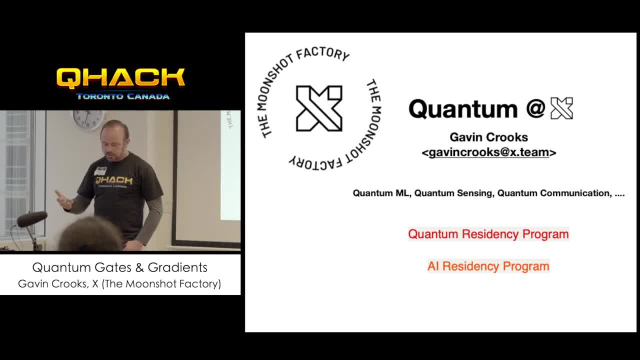 a residency program. If you're a PhD student, you can come to X for a summer, like three months, and hang out on a project. So there's an AI residency which is sort of generic to all of X You get embedded with. 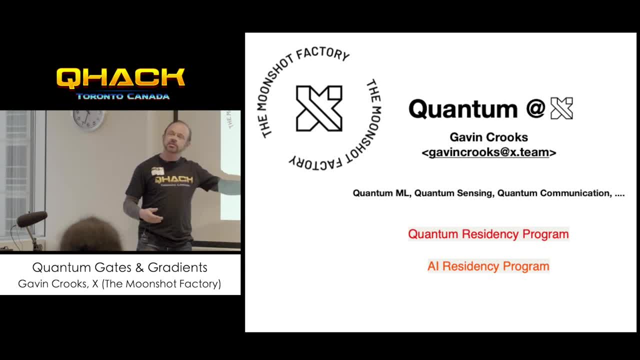 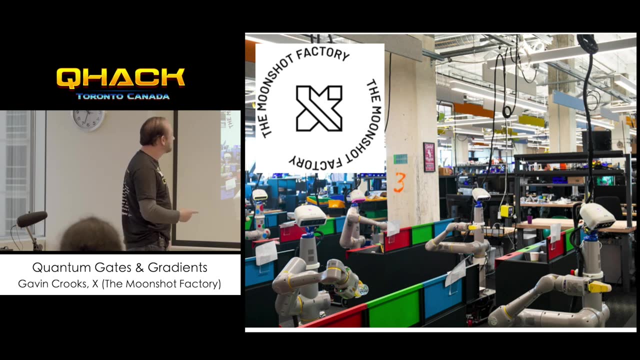 a team and do sort of applied AI. And then there's a quantum residency program that's specific to our group And this is actually pretty cool. People have come in and actually started up real projects which are now ongoing at X And oh yeah, so this is what X actually. 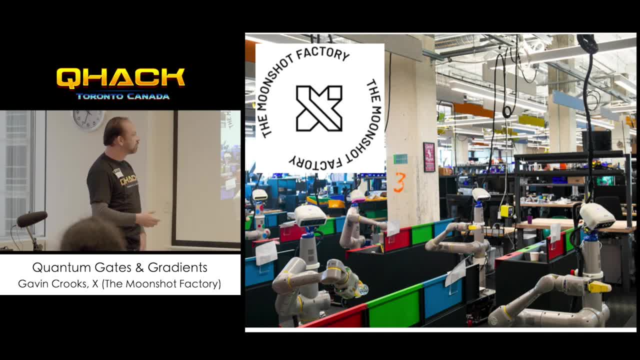 looks like. This is a picture that was published in Wired a couple of days ago, so I can show you this. This is public. This is. This is like one floor down from where we are. Where I am is fewer robots. 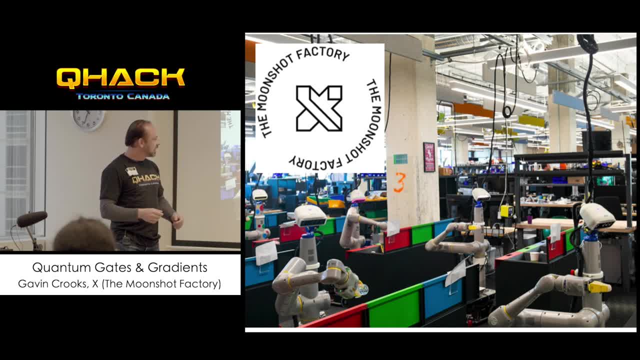 So this is like the latest project out of X that we go public Announced. It's still part of X. These robots trundle around and they sort trash, so they're using reinforcement learning to try to learn how to do useful things for us. So things that have come out: 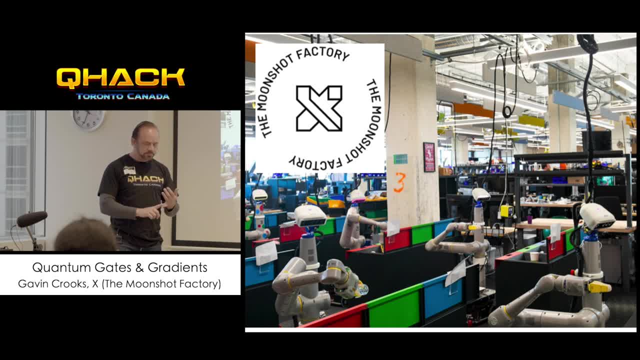 of X is like Google's startup incubator. So Waymo, the self-driving cars, was an X project. Google Brain was an X project before getting folded into Google Research. More recently there's been like Loon, which is internet by balloons. So lots of really. 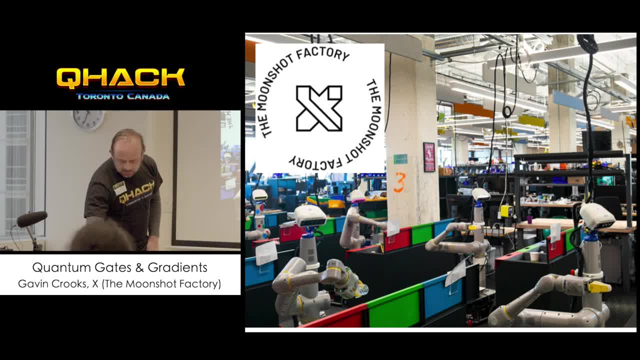 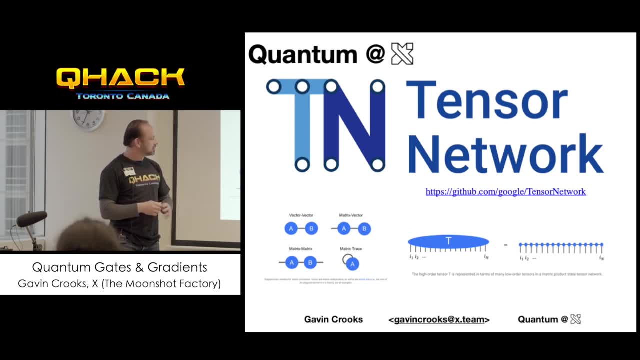 really cool stuff going on And I'll also just advertise from our group one cool thing. this software package called Tensor Network, So a Tensor Network lowercase is a network of tensors. It's a tool that came out of sort of quantum chemistry. 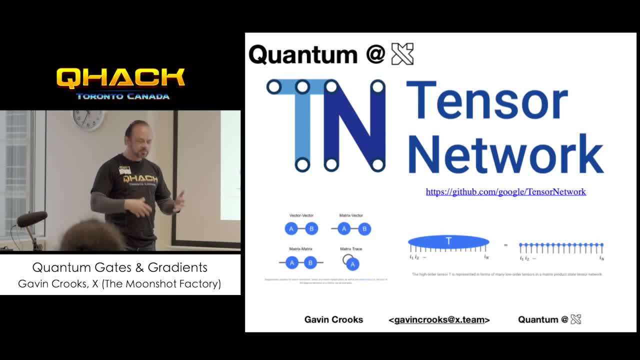 You want to do calculations of properties and materials, And so you think of diagrammatically. a vector is a blob of one leg, A matrix is a blob with two legs. A multivariate tensor has many legs, So, like a quantum state, you can think of it as a big tensor with each. 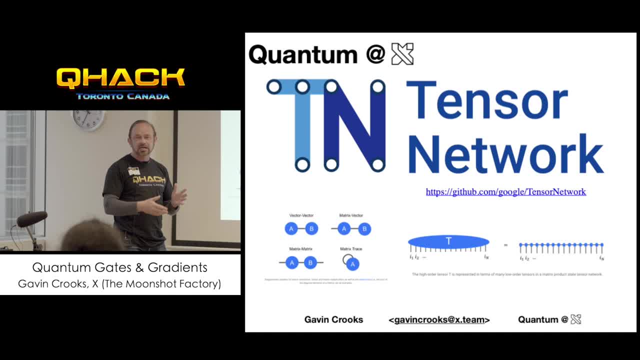 leg as a qubit, And so a quantum circuit is a tensor network. It's a simple example, And this software is designed to make it easier to build these networks. And of course it's really cool And it takes care of the back end optimization, numerical optimization. 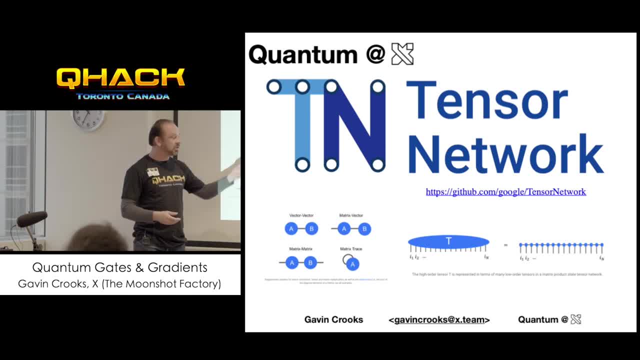 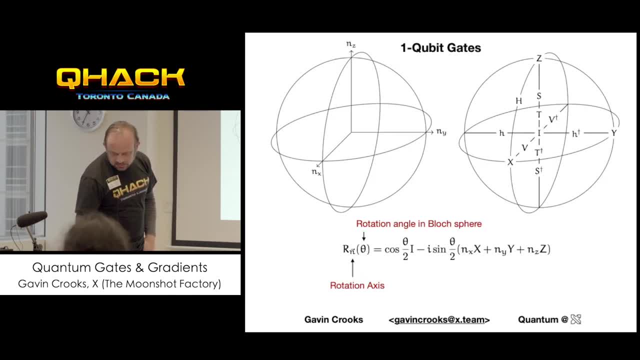 You can run these things fast on GPUs and even TPUs. Okay, So I thought today I would just talk about something old, Because- why not? I thought I'd talk about the space of gates. This is what I'm Most of what I'm going to talk. 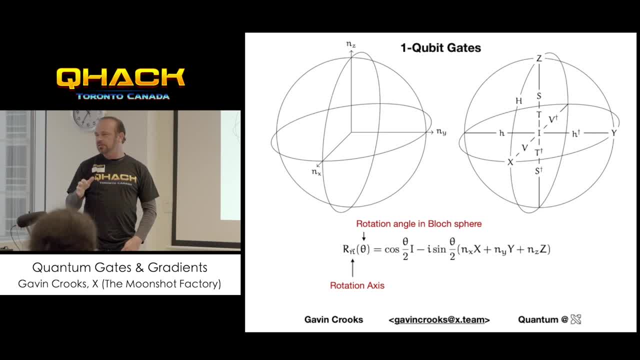 about is sort of dates, A lot of it to sort of This is sort of the mid-2000s, Really useful stuff. I think everybody should know this. It just didn't make it into the standard textbooks Because the standard textbook got written. 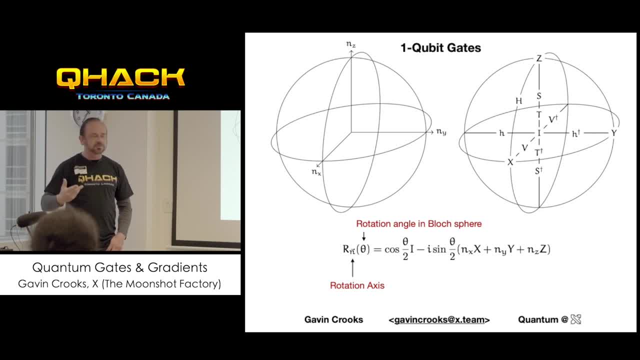 before this was figured out, So I sort of evangelize it. I think this is a really good thing to try to understand, Because as you look at these quantum algorithms, as you look at people's different hardware, you're going to run into lots and lots of different quantum. 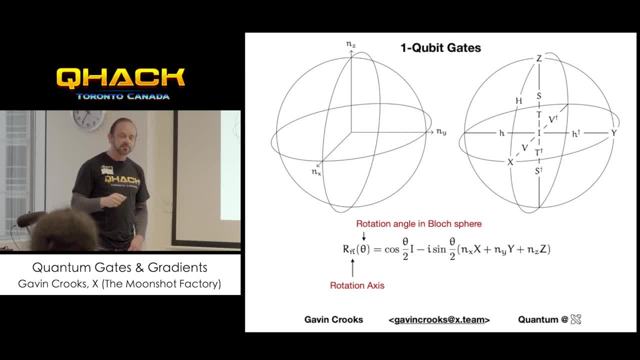 gates And it's hard to keep them all straight and how they interrelate to each other, But in fact they have a really But in fact they have a really simple mathematical structure which makes it really easy to sort. 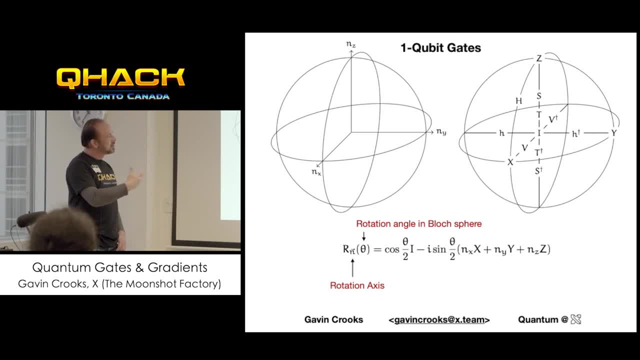 of keep track of them. So I'll first sort of give the example of one-qubit gates, But the more interesting case is two-qubit gates. So for one-qubit gates, you know, we have this block sphere. The block sphere is a way of keeping track of states, quantum states. So every point, 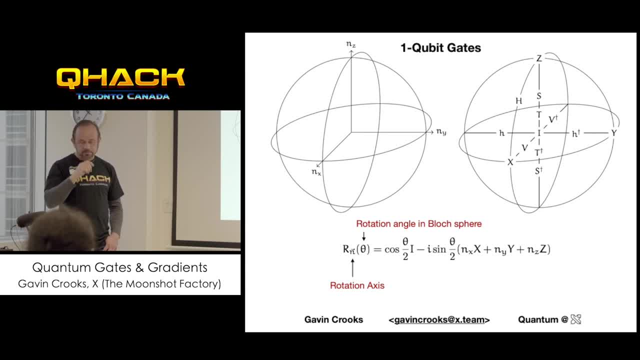 in the sphere represents a different quantum state of one qubit. So this is the same sphere mathematically. But now it's the sphere of gates. So any one-qubit gate you can write in this form: where there's some vector, some angle that you rotate about in the block. 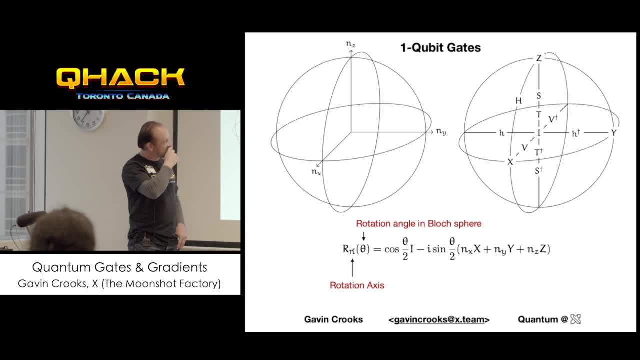 sphere and some vector in that block sphere, And so every gate, any one-qubit gate, can be presented as a point in this sphere, And it's like the block sphere- opposite sides of the sphere glued together. So X is here. 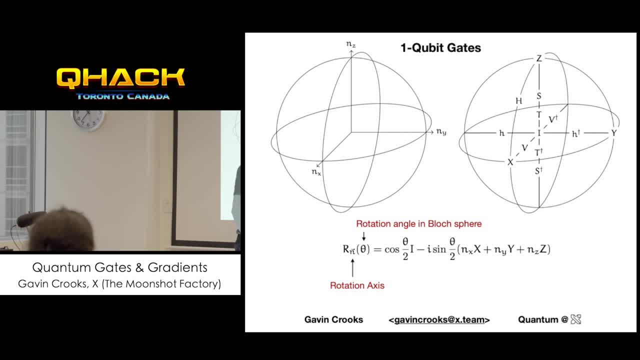 here on this x-axis. x is also here, y, y, z, z, And then all our other one-qubit gates we're familiar with just plop out on this sphere. somewhere Right in the middle is the identity gate. s is the square root of z, so it's halfway down. 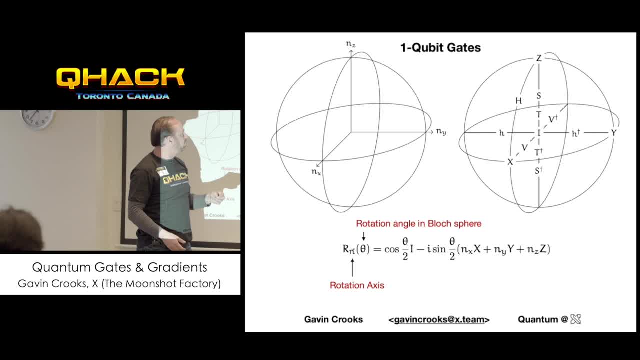 t is the square root of s, halfway down from there And then less commonly, but they still you run across sometimes. v is the square root of x. This h is called the pseudo Hadamard And the actual Hadamard is up on this axis. 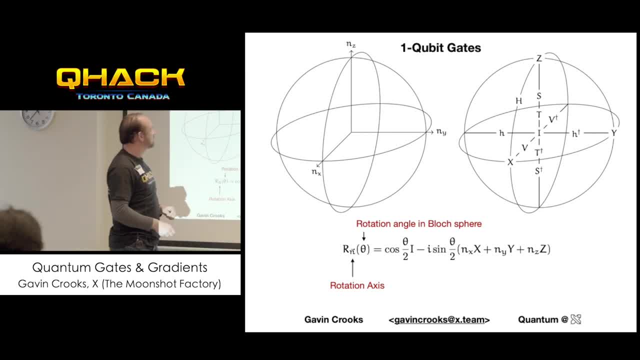 here on the edge of the sphere between x and z. So it's just a way of keeping track of this set of gates. one-qubit gates- OK, that's fine, but what about two-qubit gates? So the problem is that a two-qubit gate- 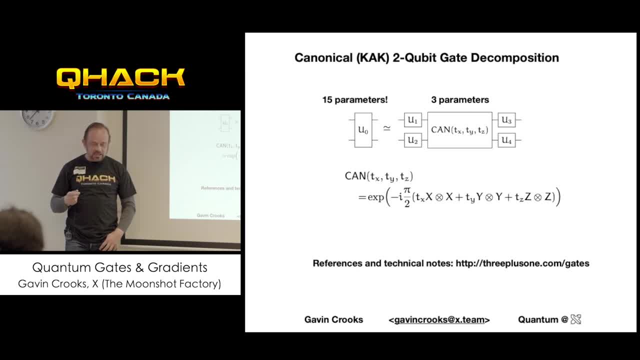 has lots of parameters. So a two-qubit gate is a 4 by 4 unitary matrix And that has 15 free parameters. The way to keep track of this is that for unitary matrix you get one parameter for every entry in the matrix. 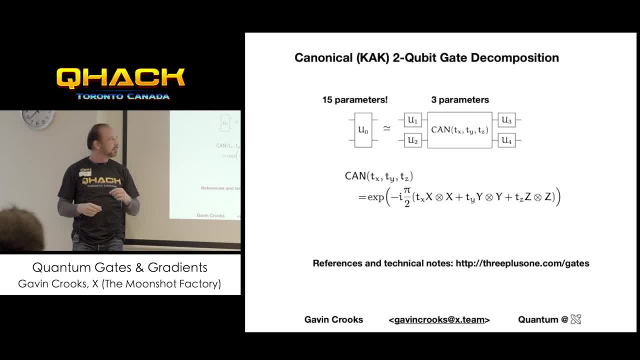 But then you lose one because you don't care about phase. So 4 times 4 minus 1.. So that's 15 parameters. That's a big space. That's too much to keep track of. But, as it turns out, what you really care about, 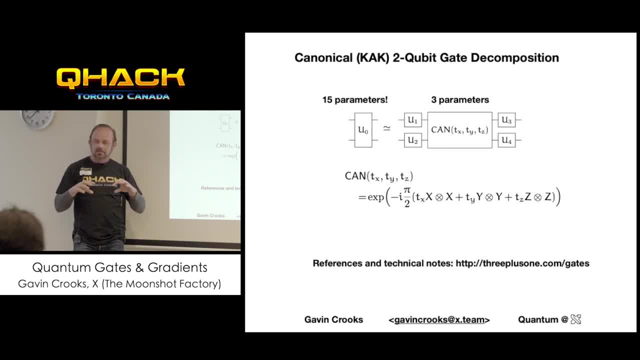 when you think about a two-qubit gate, is that sort of two-qubitness, the non-local part? That's the interesting part. There's this less interesting part. There's this less interesting part. There's this less interesting part, which is the one-qubit bit. 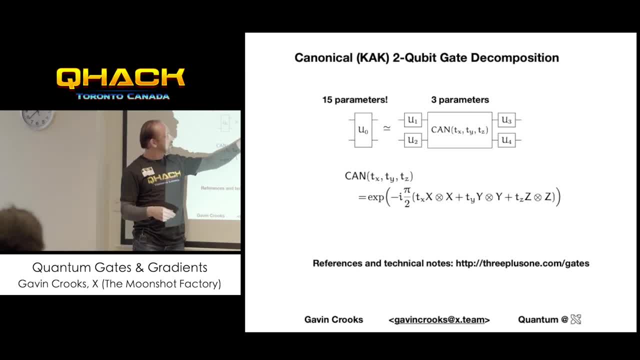 So I can rewrite this 15-parameter gate as this gate, two-qubit gate and a bunch of one-qubit gates. Each one-qubit gate is free parameters. So what I'm left over with for the two-qubit gate is just free parameters. free parameters I can keep track of. 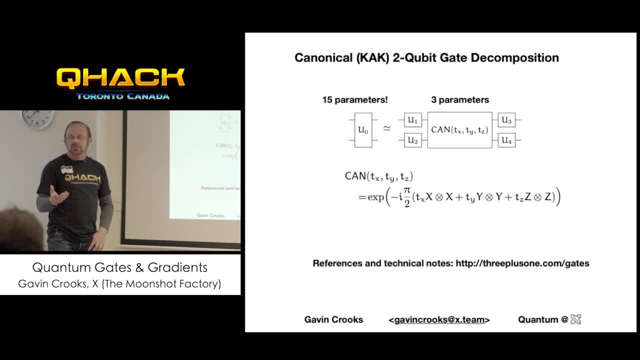 So you see, this called the KAK decomposition, because that was just the notation that was used in one of the original papers, or the canonical decomposition. So the idea is you take any two-qubit gate, take out the local parts, the one-qubit gates, just leave behind. 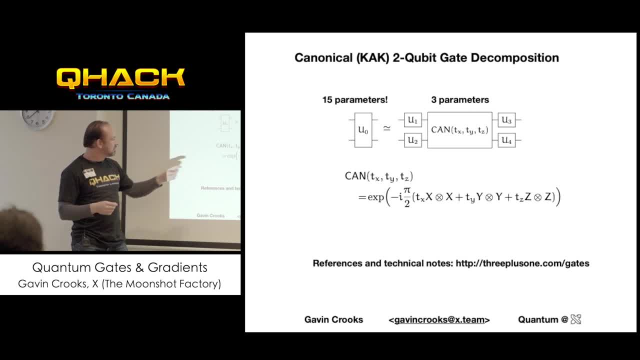 this interesting two-qubit bit, And mathematically it just comes out like this: You have poly, xx, yy, zz and one parameter for each. So the space then turns out to be a cube, So instead of being a sphere, this time. 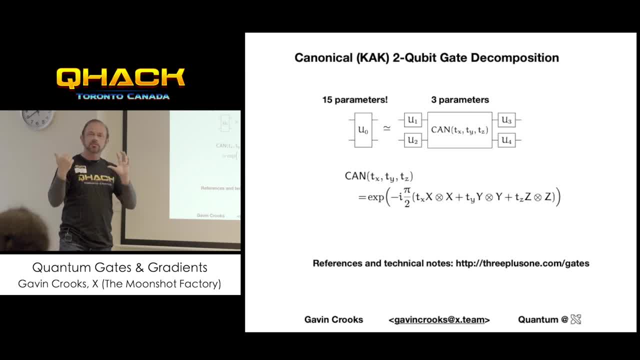 it's still three-dimensional. This time it's a cube, And you go off one edge and you come back in the other. So it has the topology of a torus, But then it turns out to be lots and lots of. for some reason, 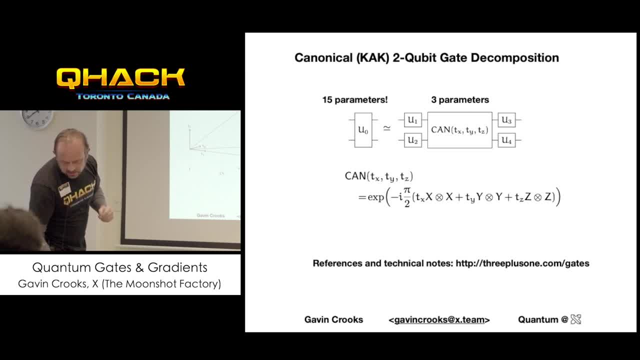 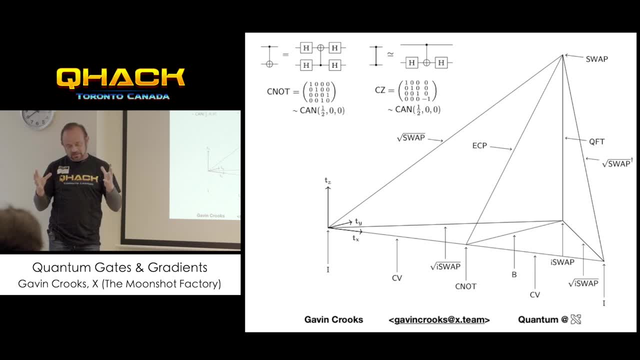 my fingers moved. No matter, I'll just skip to the next slide, which has it in the right place. There we go. So it turns out there's lots and lots of symmetries, And to remove that I'm going to do this. 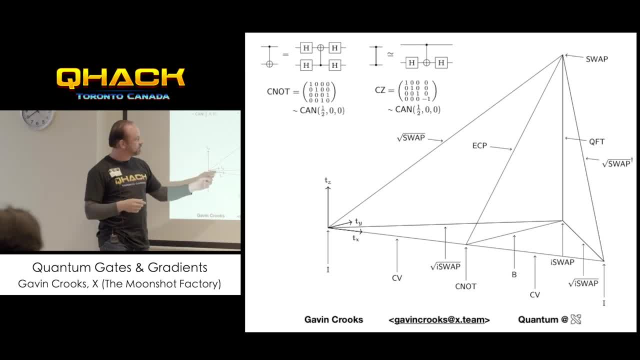 To remove all the symmetries. instead of a cube you get this sort of pyramid shape. All our favorite two-qubit gates are represented by some point within this volume. So the x-axis is this way, y-axis is that way. 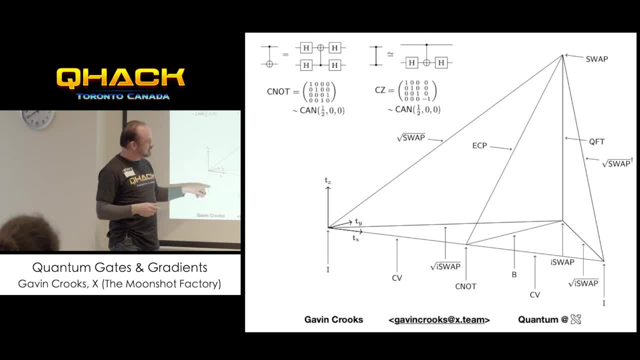 z-axis is straight up, And so where's our favorite gates? Well, the identity is here, And then there's a symmetry, So it means it comes up on the other side. This x-axis, you get c0 right here. Iswap is at the back corner. 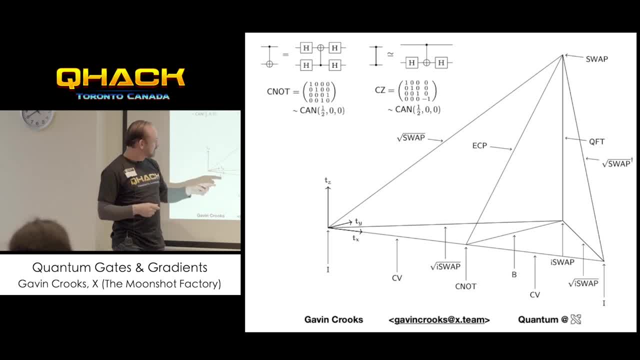 Swap is at the bottom, Swap is at the top, And then we get things like the square root of swap Turns out. this is like half a unit, one unit, half a unit up. So there's interesting gates at every quarter unit. 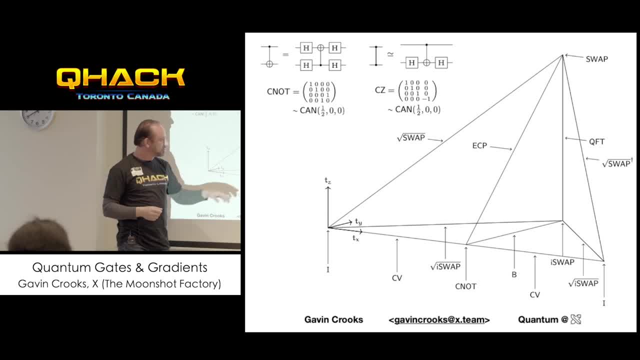 So this is the square root of c0, square root of iswap. There's only one square root of iswap. Again there's a symmetry. It looks like there's two, but again they're related by local transformation. So who cares? 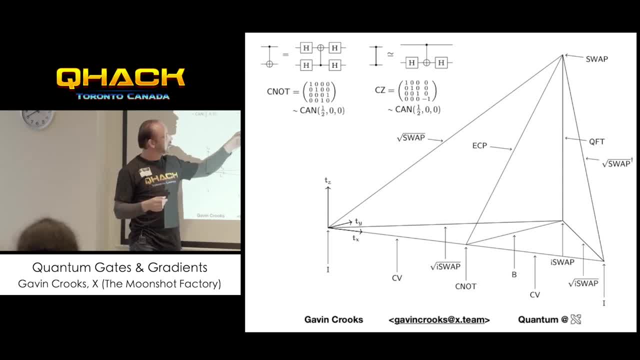 There's really only one, But you get two Square root of iswap, And then at the back edge over there, there's the quantum Fourier transform, And what else do we have? Oh, this is called the b-gate, which is short for Berkeley. 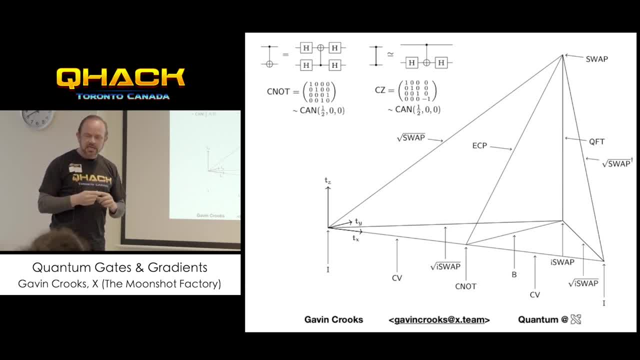 Turns out that was a gate that was investigated because it has the interesting property that you only need two b-gates to make any two-cubic gate. So you want to make any two-cubic gate, you need three c-nots. Two c-nots gives you any gate in the bottom plane. 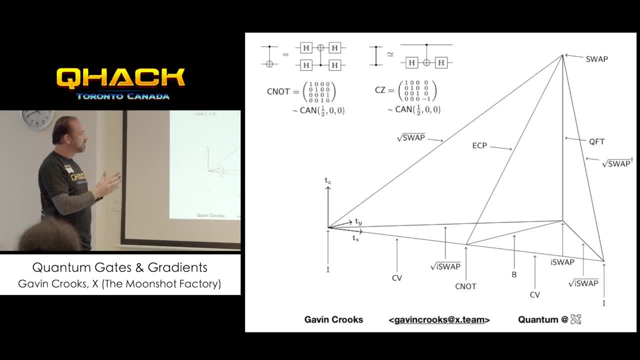 Three c-nots you can get any gate in. the whole volume Turns out with a b-gate. you only need two b-gates. But it's not a natural gate, So it doesn't turn up often in actual hardware in that sense. 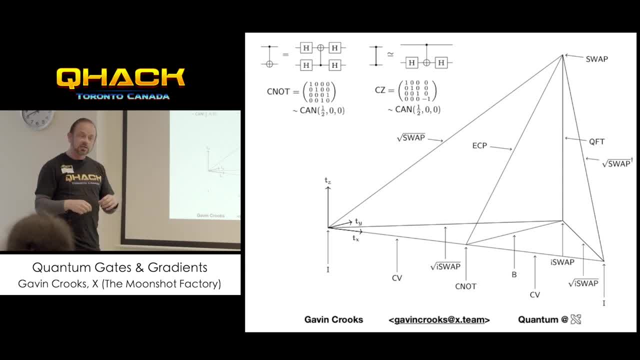 And this helps you keep track, I think, of this plethora of gates, because there's lots of gates you'll run across which are really just repeats of the same gate. So, for example, c-not is really the same as cz, because you can transform one into the other just. 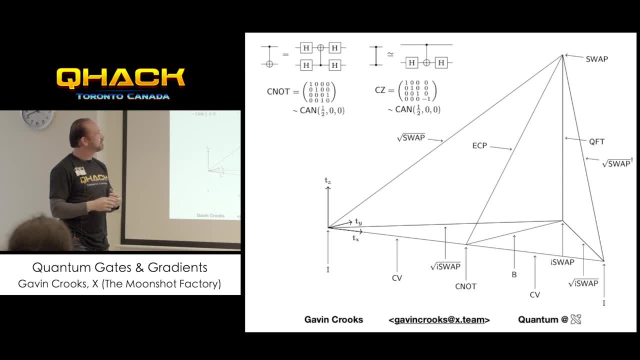 with local gates And typically in a lot of these cases hardware platforms, it's the two-cubic gates that are the expensive ones And the one-cubic gates are relatively cheap and low error. So the difference between c-not and cz it's not that big. 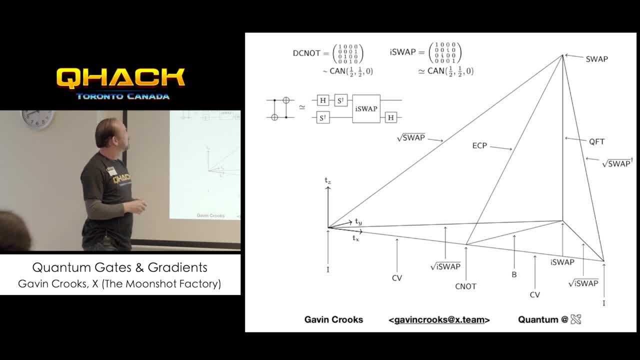 And another one I like is the double c-not. You run across this in circuits lots of times. Two c-nots back to back is actually locally equivalent to an I-swap. So again it gets you on that back edge, this back corner. 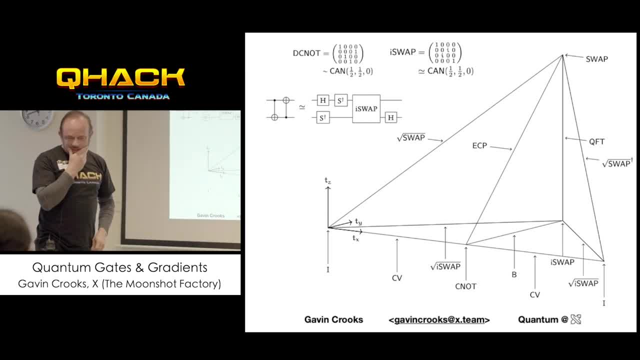 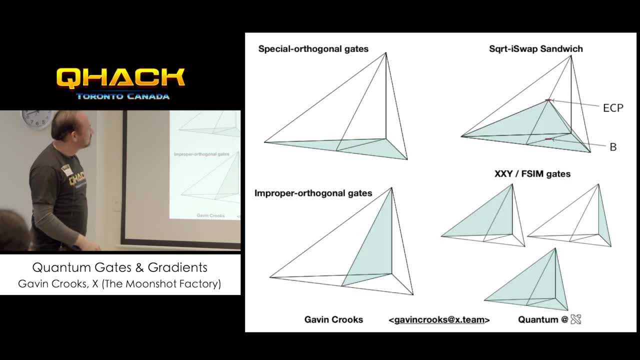 over here. So all of the planes in this volume edges and planes have meaning. So this bottom edge is the one that's going to be the bottom. So this bottom edge is the one that's going to be the bottom. So that's the surface. 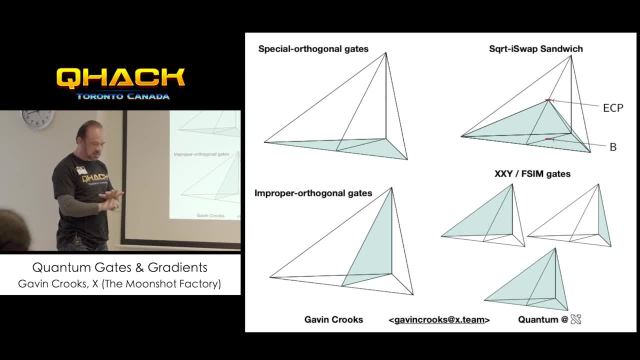 It's that surface that you can get from two c-nots And those turn out to be the orthogonal gates. Those are the gates you can represent locally, up to a local transformation by a orthogonal matrix. So these ones are the special orthogonal gates. 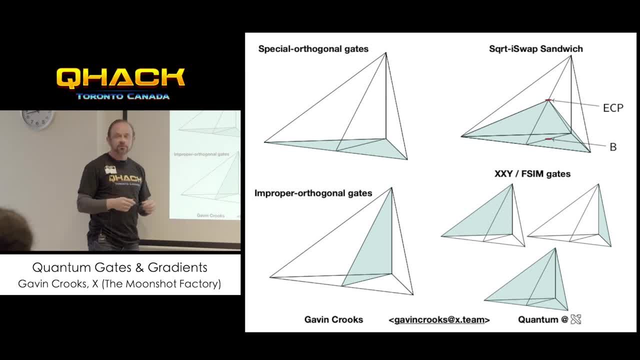 They have determinant 1.. These ones, this way, actually are the improper infogonal gates, which is the one the infogonal gates will have determinant 1, minus 1.. And then you have voids, Volumes 2.. So there's a little pyramid here. 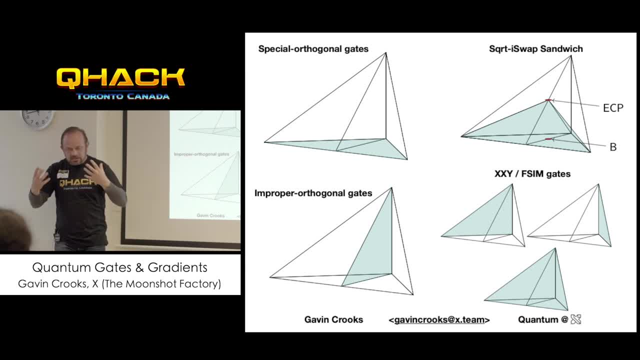 Turns out if you take. you know, as you try to design the quantum circuit, you look at the repertoire of gates that are available in your hardware and you ask, well, what set of interesting gates can I get out of this? So it turns out the square root of I-swap in some setups. 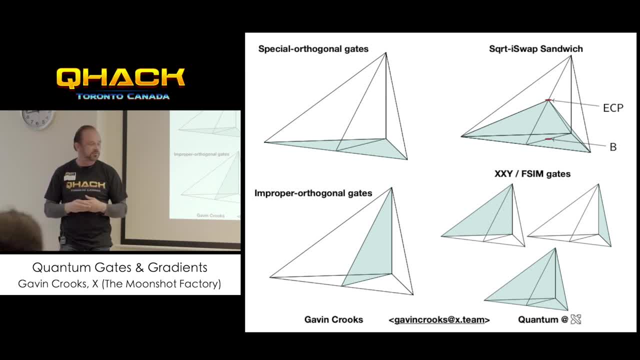 might be a natural thing, a gate for some of these hardware platforms. What if I have a sandwich with two I-swaps And you ask: what set of gates can you generate out of that? So with two CNOTs you can only get that bottom plane. 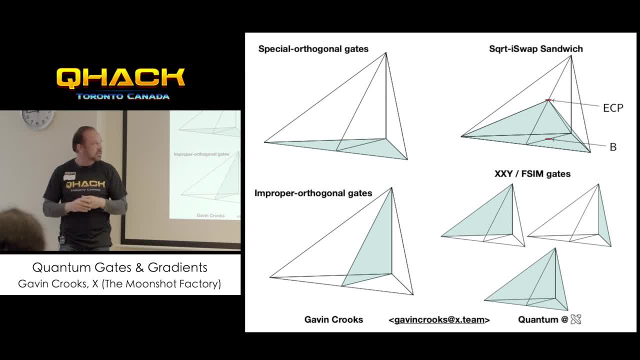 But with two square root of I-swaps you get this little pyramid of gates, And the B gate there is in the bottom, middle, And this gate at the top is what I call the ECP gate, because it's the only point in this thing that 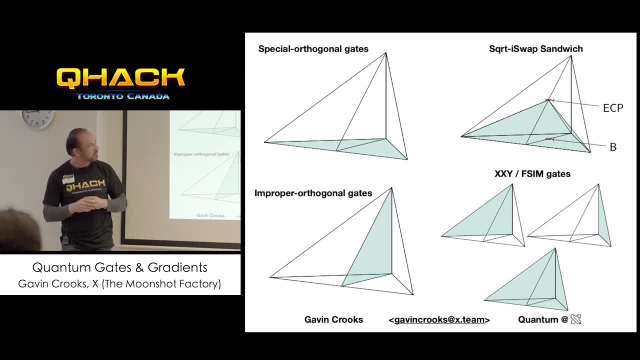 doesn't seem to have a name, So I call it ECP, which is named after someone who works at the gate- OK, Our compiler guy who sort of figured this out originally. Oh and then again, this sort of helps you understand the different hardware platforms. 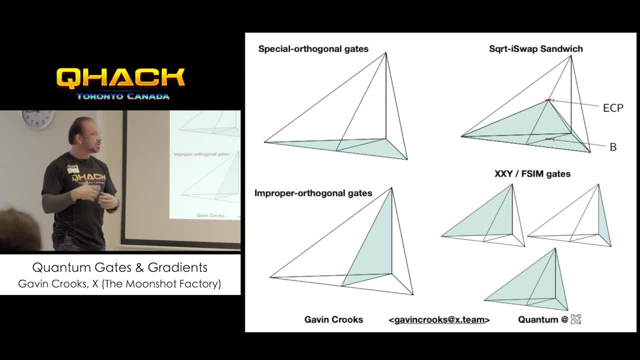 So Google's new Sycamore hardware platform has sort of a natural gate, what's called in CERC F-SIM or elsewhere you see called XXY, And this is a gate with two parameters. It turns out what that represents. 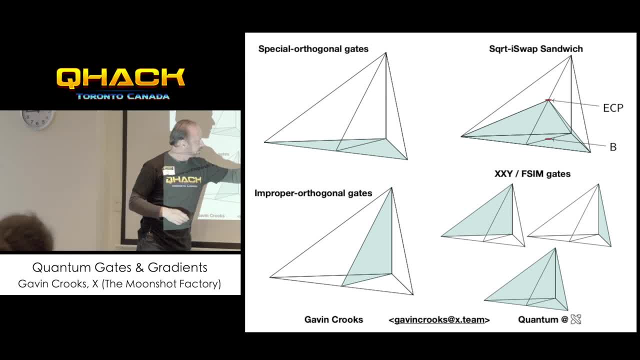 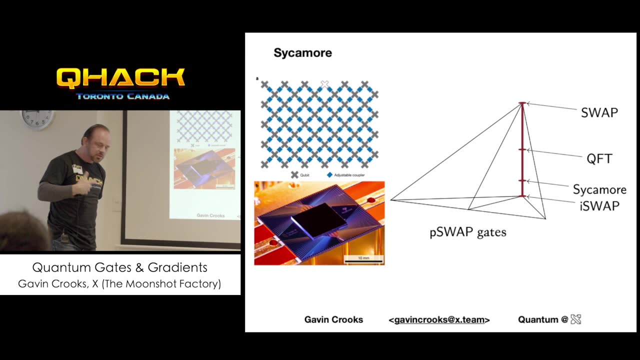 is the top three faces of this pyramid. so one, two, three faces. You can get anywhere in those three faces in principle with this F-SIM gate, But again, as we design algorithms or circuits for these near-term machines, everything is so noisy. 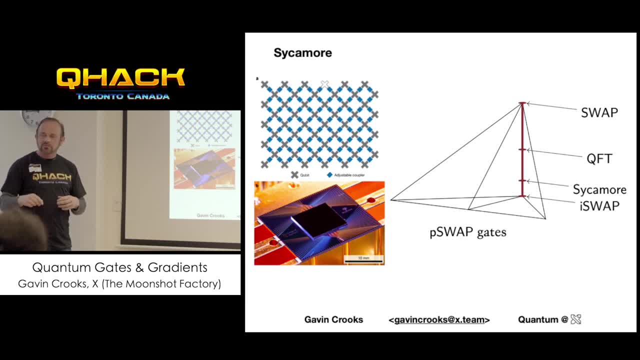 we have a very few gates we can get away with. So you really need to design to the hardware, You need to try to use the natural gates of that particular hardware And for the reason that I'm talking about, I'm going to go. 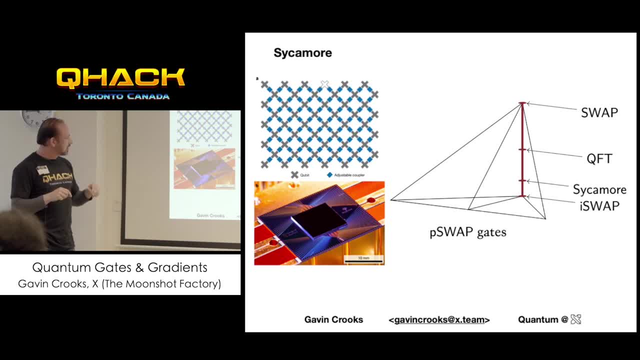 over this. This is the Sycamore chip that Google did the supremacy experiment on recently, which I agree is a terrible term because it's not supreme right, It's not a useless program, It's a useless, It's a supremacy. 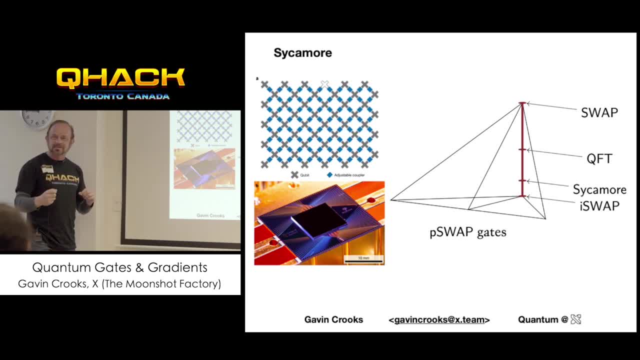 You know, air supremacy, right Second World War, means that you dominate in every possible way, whereas this means that the question if you want a computer can do one problem better than the classical computer. But it's good marketing, right, I guess. 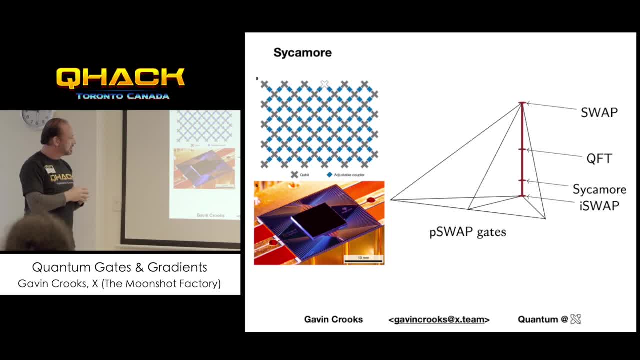 But whatever, It's still a good. you know we should celebrate it. It's a milestone, But it's still a long road to go. Oh OK, So turns out, for this chip they actually tuned up one particular F-SIM gate. 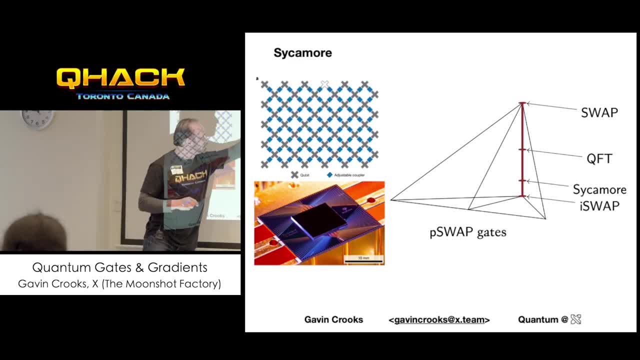 And it turned out the one they tuned up is on this back edge. This back edge actually is called PSWAP in PyQuil, Did you? where did that come from? That's the only place I know it from Frametrized swap. 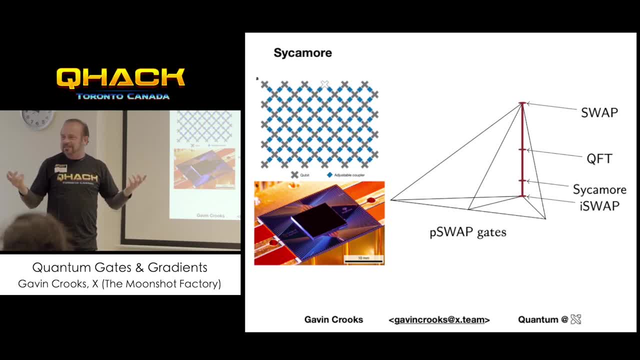 Yeah, that's what it stands for, But do you guys just invent it and be cards, I guess. so, yeah, Yeah, yeah. So the only place I know this thing is from PyQuil. We may have a lot of reasons. 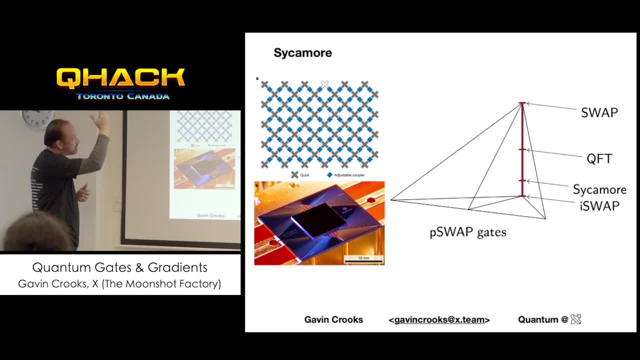 Yeah, yeah, no, no, that's cool. No, no, no, Because it was. yeah, it turned out to be this back edge, And this back edge didn't have a name apart from PSWAP, And so at the top is SWAP and at the bottom is ISWAP. 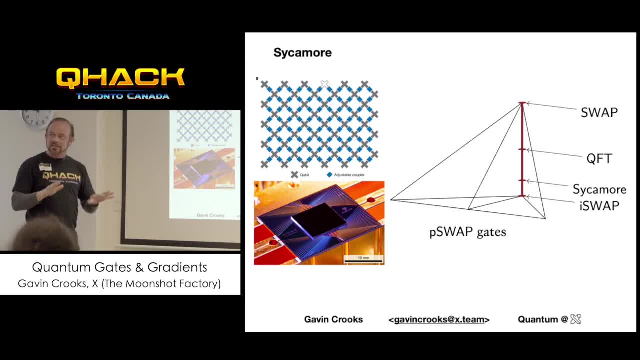 In the middle is the two-qubit quantum Fourier transform. It turns out this Sycamore gate is kind of weird. It's one-sixth of a way up this back edge And the reason is just because of where the hardware worked out that particular parameterization. 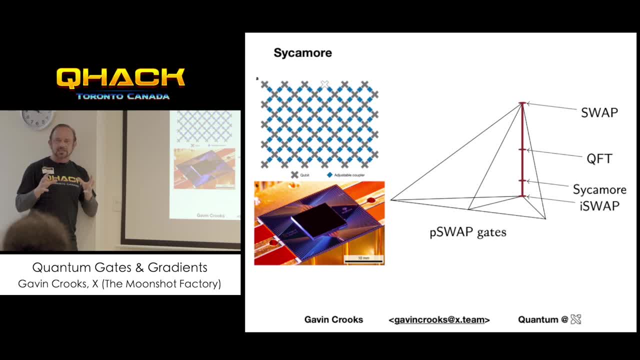 the gate is really fast. And if it's really fast it also means they can make it relatively low noise. So it's the natural gate for this particular hardware system. It's not the natural gate. if I want to start just thinking about, well, quantum circuits, I'd 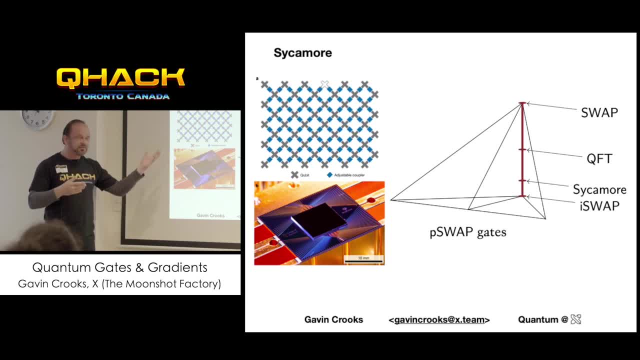 start with CNOT or something, But it's the natural gate for this particular hardware. So therefore, again, you need to understand what these gates are, And it's a sixth of the way up this back edge. Compiling to this is actually kind of interesting. 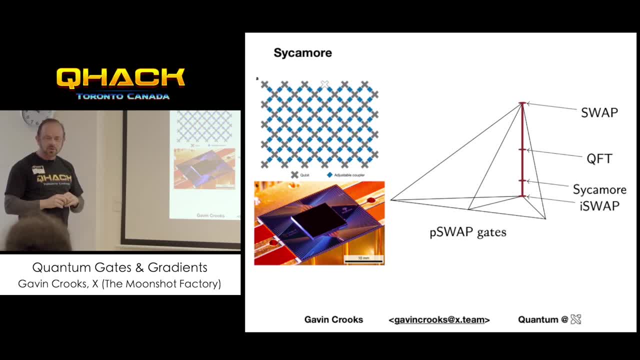 Yeah. Yeah, It's interesting There's just keeping a watch on the circ, pull requests, So what they're doing is the Sycamore- well, that's the ideal Sycamore gate, But in practice every point in the circuit. 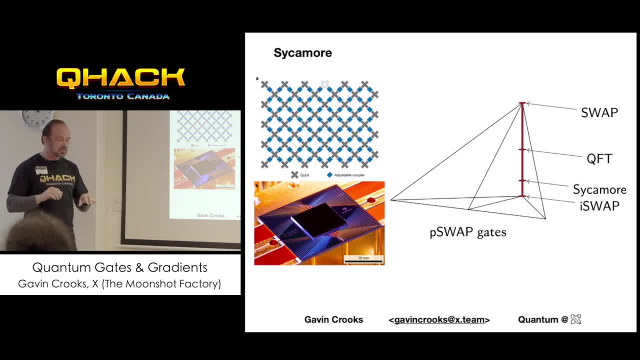 is actually getting a slightly different gate with slightly different parameters, But it turns out what you can do is you can line up two Sycamores as a sandwich And you can build that B gate. I was talking about the Berkeley gate, And two Berkeley gates will give you any gate in the circuit. 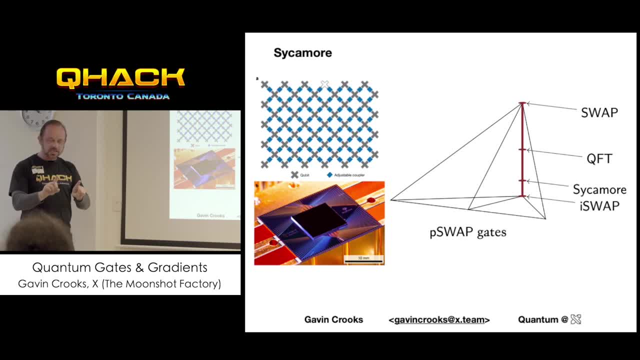 In the pyramid. So they know how to take two Sycamores and turn it into a B gate. You know how to make any gates in this pyramid out of two B gates, So therefore you can actually compile to the Sycamore gate. 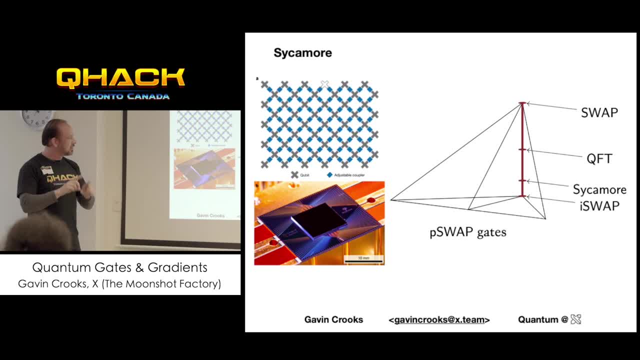 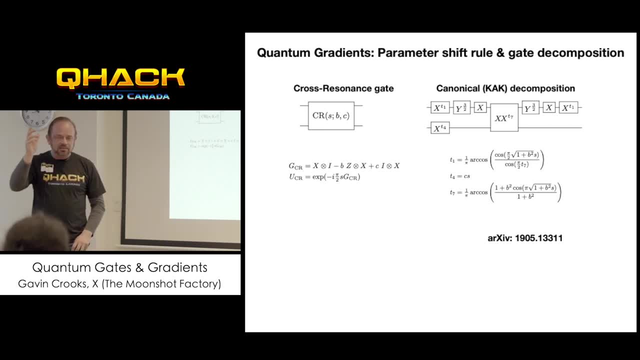 even though there's this variation in the points. Great, Well, I mean. OK, I was only going to touch on quantum gradients. So one of the other useful things here is this parameter shift rule, which is a really, as Maria was saying, a really neat way. 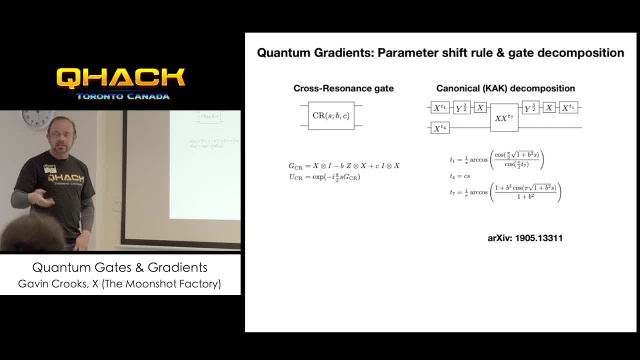 of being able to take gradients of these quantum circuits and therefore being able to do gradient descent and try to optimize these circuits. But this parameter shift rule has this requirement in it that the structure of the gate, of the Hamiltonian of the gate, 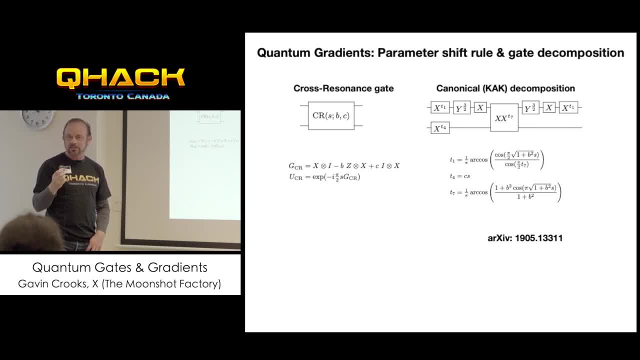 has to have this particular structure to it And at first sight that looks like it's restrictive. Turns out, it's not Turns out. you can always recast any gates. OK, Into a gate that you can do. parameter shift rules on. 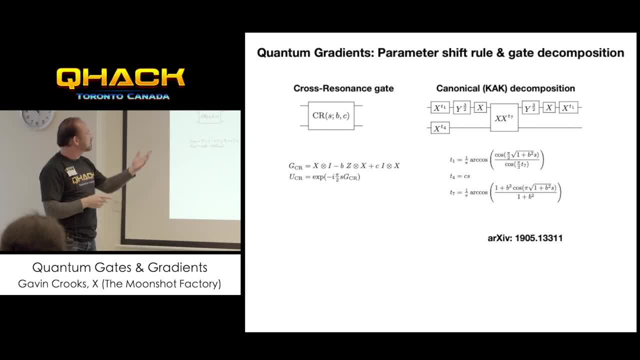 So this is a particular example I worked out just as an exercise. So the cross-resonant gate is something that's natural for certain superconducting qubit hardware. It has this sort of structure of a bunch of parameters And you can't directly take the parameter shift. 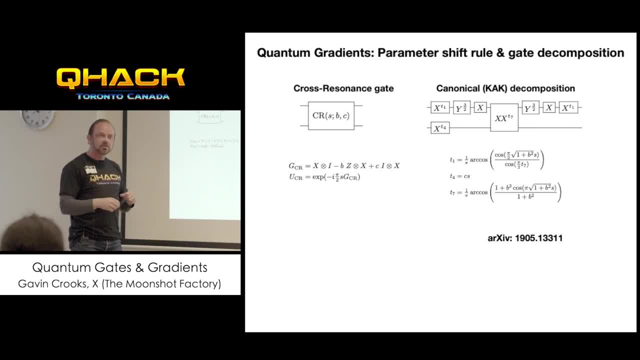 rule for this gate. But you can decompose it. If you can decompose it into other gates, you can take the parameter shift rule of, you can take the parameter shift rule gradient of this whole gate. So it turns out the full decomposition of this thing in the canonical decomposition. 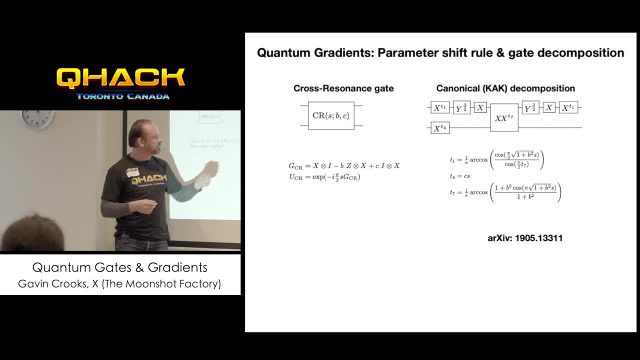 gives you this bunch of stuff, And then it turns out to be horribly complicated with some not simple math, But it's doable. So in principle we can always apply this parameter shift rule. We might have to jump through some hoops to get it to work. 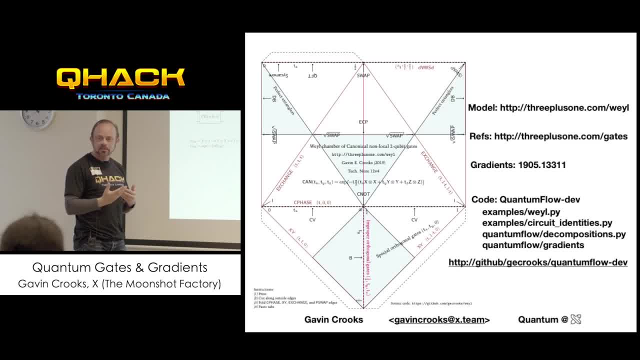 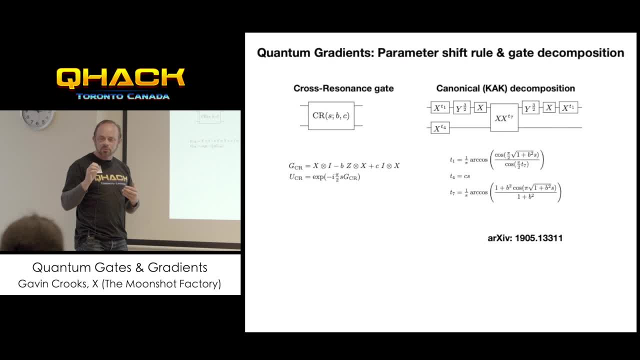 But it's a really powerful way of thinking about gradients. But just to reiterate some of the questions that came up last time, it absolutely is an open problem about the right way to optimize these quantum circuits. Problem with the parameter shift rule is that you get out one gradient at a time. 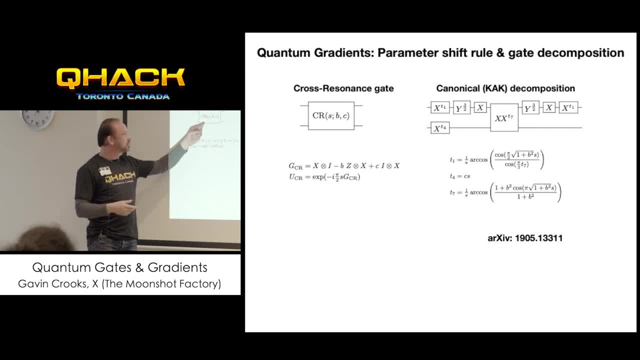 So you have to run the circuit twice. You get out a gradient of one gate And your circuit can have many gates in it, And that gradient is noisy because you're only ever going to take a finite number of shots. So is there a way around that problem? 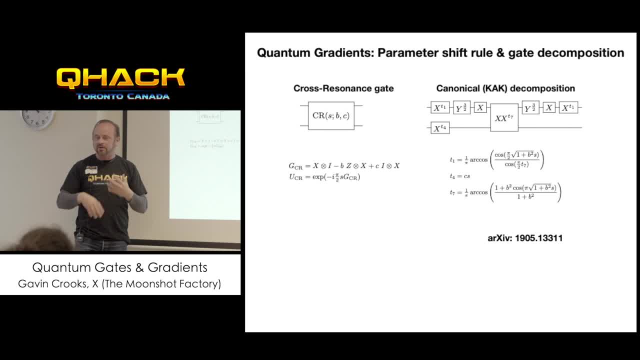 Possibly. But yeah, I think it's still very much an open problem what the right way to do this is. I mean, I've done some sort of proof of principle back of the envelope calculations that you can actually optimize some non-trivial circuits with a number of shots. 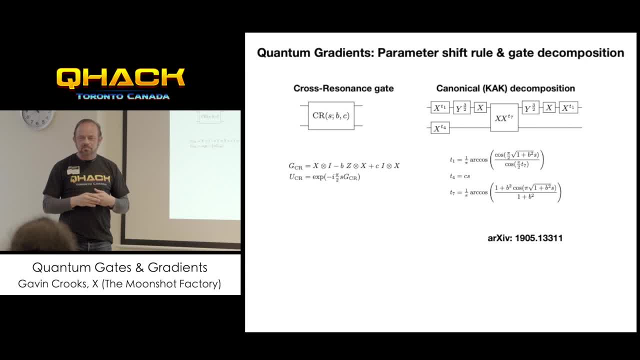 on actual hardware. that's not unreasonable, But then the hardware itself is also noisy, So there's an extra level of complication. We're going to have to try it and find out. It's very much an open problem at this point. So yeah, I'll just finish up. 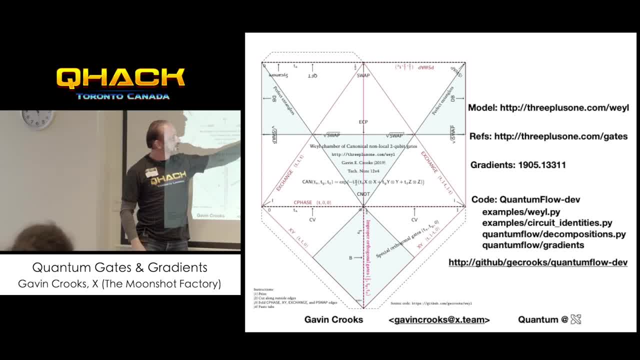 Just some links. This is my rough notes about this stuff. If you'd like to do some paper craft, there's this nice little model you can print out And you cut it out and you fold it up and you'll have your own little pyramid, just. 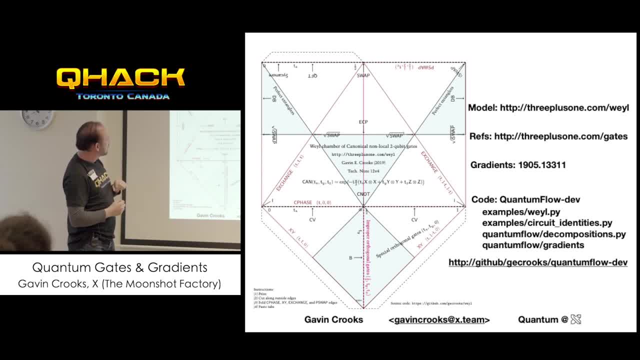 to keep track of where all the little gates are. It has a couple of extra ones I didn't mention. Some of these edges are labeled. This is the DB gate, which again my friend came up with. I forget what it stands for. 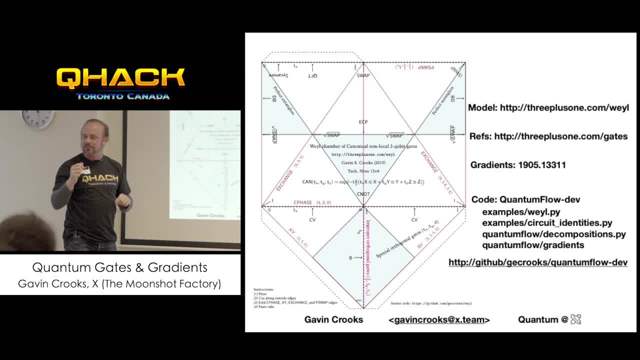 It's some weird American cultural reference. Yeah, yeah, yeah. Dagwood Bunston, Dagwood. Does it make any sense? I don't know, Huh? Dagwood Blondin? Yeah, maybe Because it makes really big sandwiches. 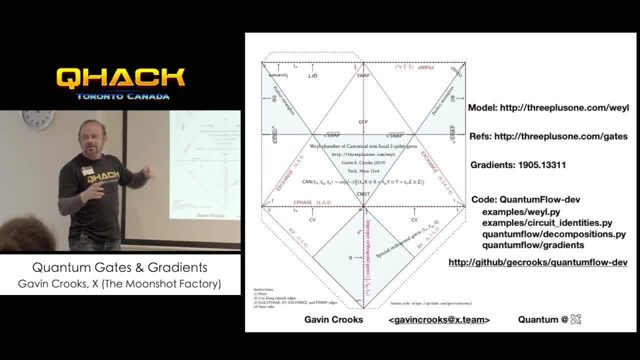 Yeah, Dagwood, Yeah, OK, Yeah, yeah. So it turns out, if you take any of these gates on this back edge, which might be generated naturally in certain hardware platforms, and you sandwich two of them up and ask: what set of other gates can I get? 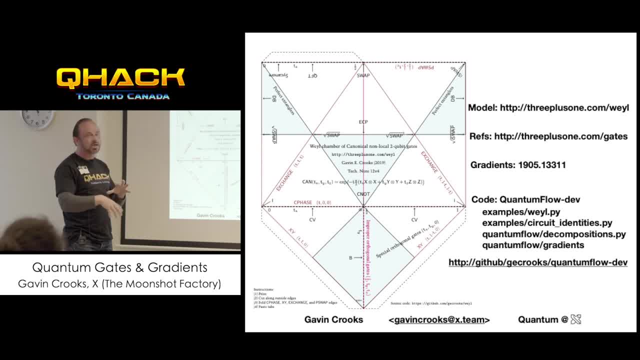 you get quite a lot with the Swearer and iSwap, but sort of the best one in terms of the biggest volume of gates you can get is this DB gate And I wrote a paper on gradients. There's Penny Lane. This is actually where I learned about this whole stuff. 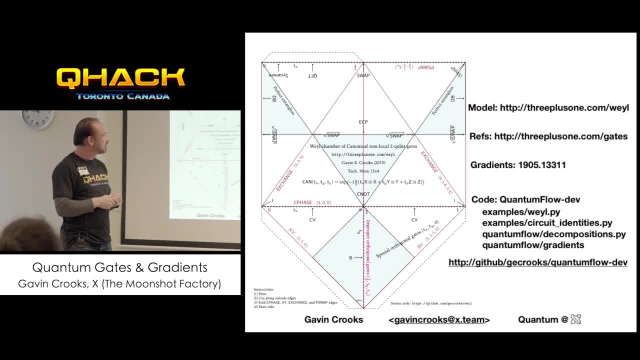 It's from the Penny Lane software. It's really good for this stuff, for the gradients. But I have some other stuff. I have some of my own example code And this lets you do this: explore some of these issues with looking at these space of gates. 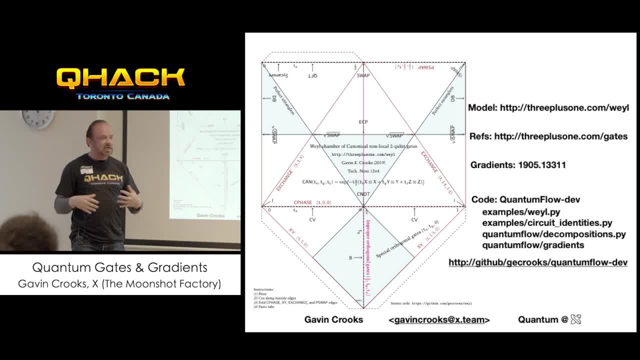 So again, this is all actually pretty old stuff. I've got lots of references in here. It's just one of those tools that should be sort of widely known because it really helps understand this plethora of gates that you tend to run into in the literature. 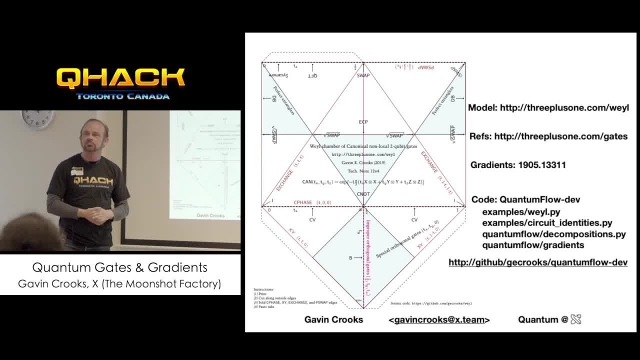 And questions. So you mentioned that it kind of suffices to consider just three parameters in order to describe any two-qubit gate in this kind of pyramid volume. But what happens to all the other one-qubit parameters? Do they stay fixed Or do they change depending on what two-qubit gate? 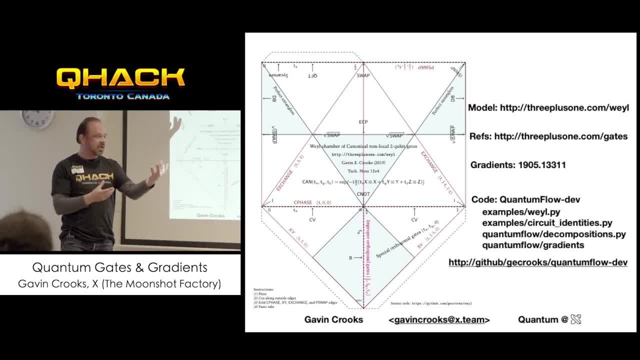 you're considering. It depends on, yes, which two. So I have CNOT versus CZ. They have the same canonical parameters, but they have different one-qubit gates on the outside. So, yeah, so they're the same gate up to this local transformation.